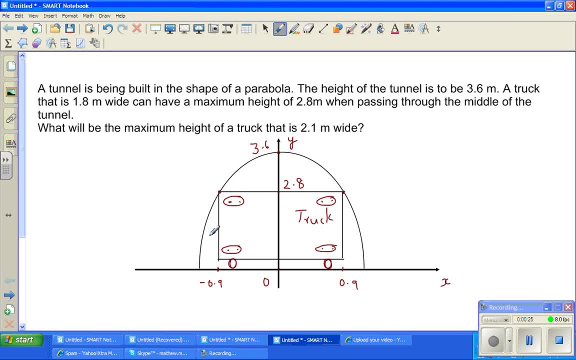 to be 3.6 meters. So this is a tunnel, So this is your tunnel. I've drawn the tunnel in the shape of a parabola and the height is 3.6 meters. Okay, so you can see, this is an upside-down parabola. A truck that is 1.8 meters wide can have a. 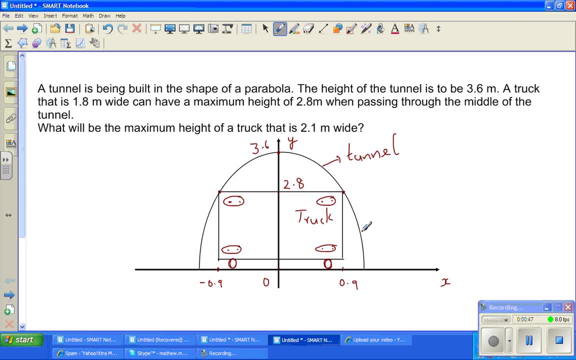 maximum height of 2.8 meters when passing through the middle. So this is the middle of the tunnel and this is say that that truck, which is 1.8 meters, So you will have negative 0.9 to the left and 0.9 to the left, So 0.9 on both sides will make 1.8 and the height is 2.8.. 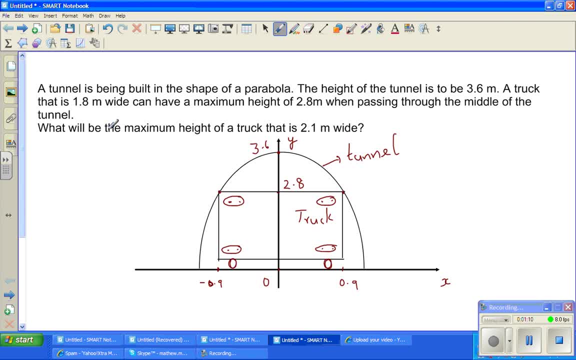 Another question is: what is the maximum height of a truck that is 2.1 meters wide? That means say, here you have say 1.05.. Okay, this is negative 1.05.. Negative 1.05 is half of 2.10.. 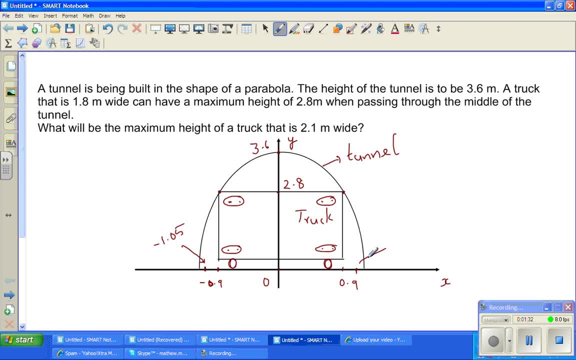 So the year you have got say positive 1.05.. Okay, Okay. so now if this the question is: if this truck becomes wider, that means it becomes 2.1 meters wide. obviously the height cannot be 2.8.. It has to be less than that, Okay. so. 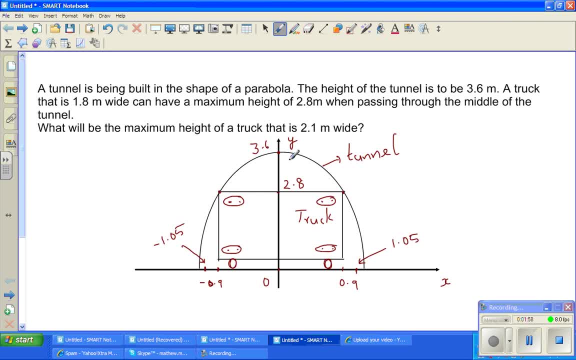 that's the question. So to answer that question, we need to write the equation in the form of this parabola. So by looking at the parabola I can see this parabola, the suppose I'm talking about. say, let me draw the graph- of y is equal. 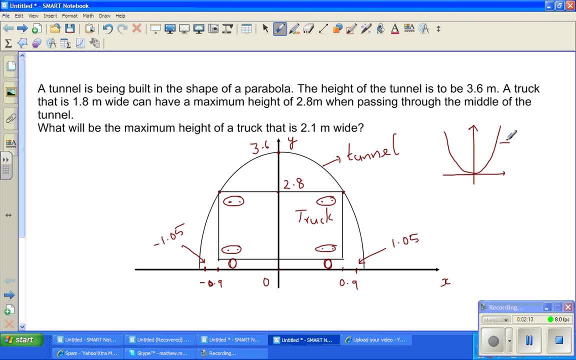 to x squared. The y is equal to x squared. This is what I'm talking about. This is the graph of: y is equal to x squared. Now, what has happened to this parabola with respect to this So well, I can say: well, this has gone flipped over, So it has. 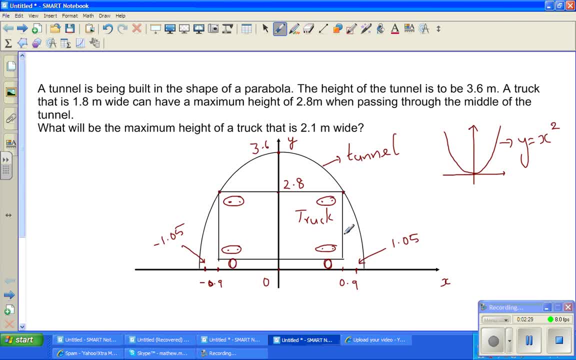 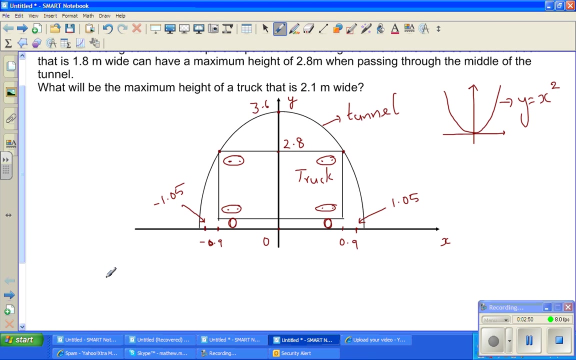 gone upside down and that is a stretch factor, Okay, and it has also moved up, Okay. so there are three transformations that are very obvious here. It has flipped over, it has moved up and there is a stretch factor. Okay, it is pulled, Yeah, pulled on by on both ends. Okay, so I can say y, Okay, 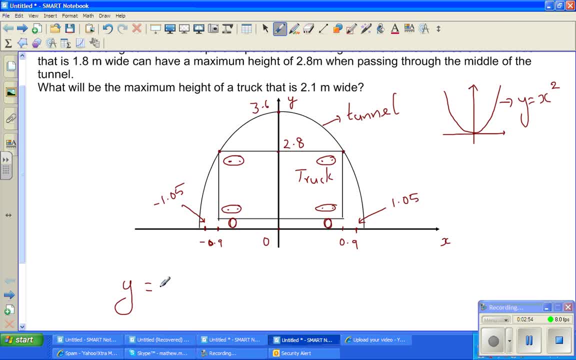 so the equation of this parabola should be: y is equal to a x squared. This parabola hasn't moved to the left or right. It has moved up plus 3.6.. Okay, now this? this will answer this. a number will tell me two transformation: This: 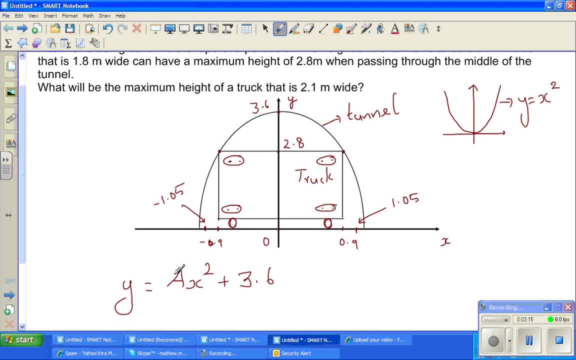 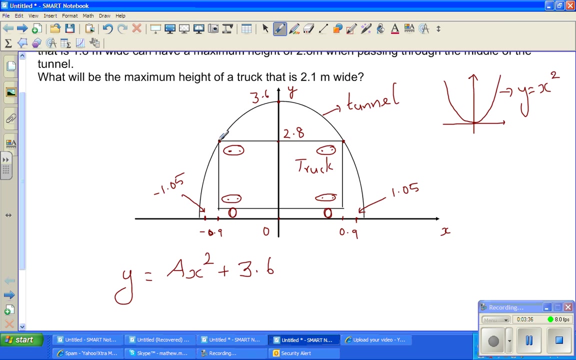 number I know should be negative because it has flipped over and as it is, as it has been stretched or pulled to, but this will be a decimal number. That's my guess. Okay, So I have to just now find a by what? So we know this point. Can we say, or let us: 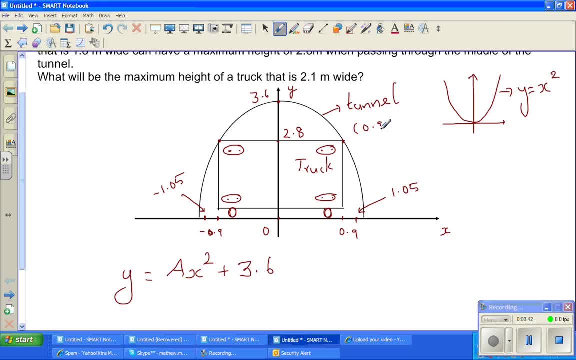 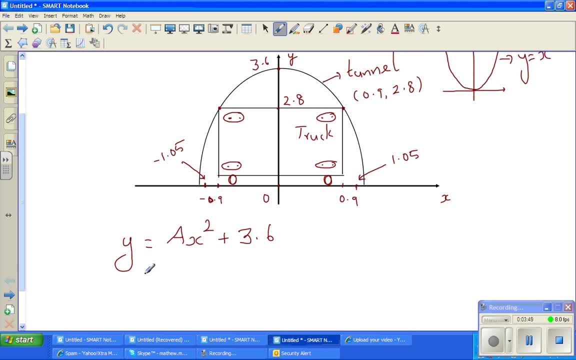 take this point. This point is 0.9 comma 2.8.. So I can put x as 0.9 and y as 2.8.. So I can say: well, 2.8 is equal to a times 0.9 squared. 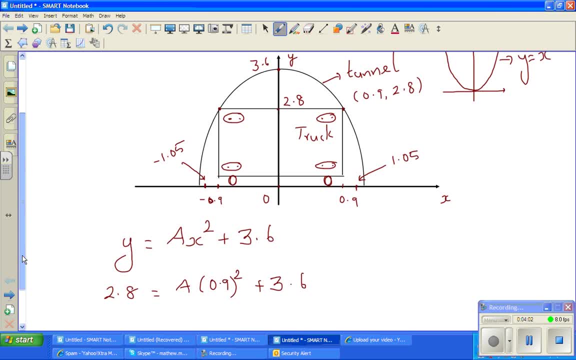 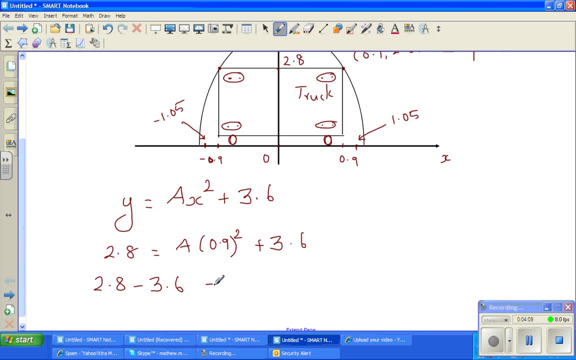 So I can say: well, 2.8 plus 3.6.. So taking away 2.3.6 from both sides, you get 2.8 minus 3.6 is equal to 0.9. squared is 0.81. a Okay, 0.9 squared is 0.. you can do this on a calculator. 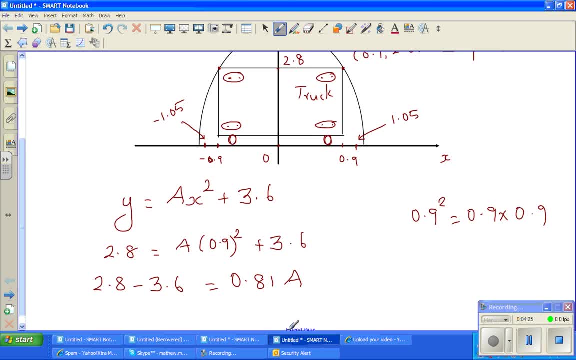 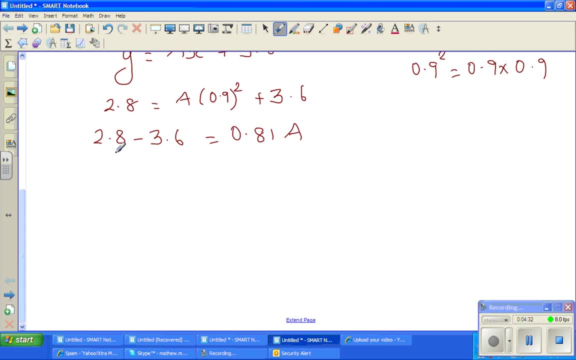 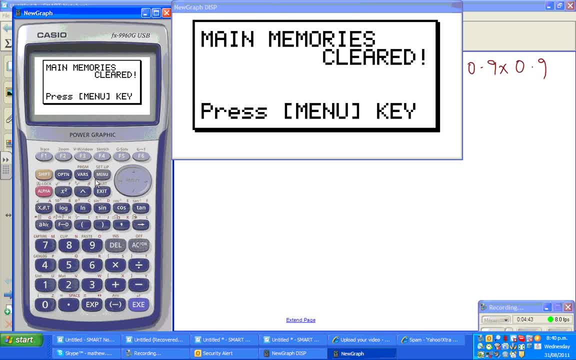 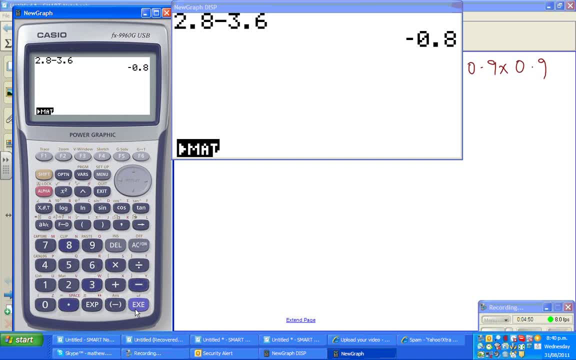 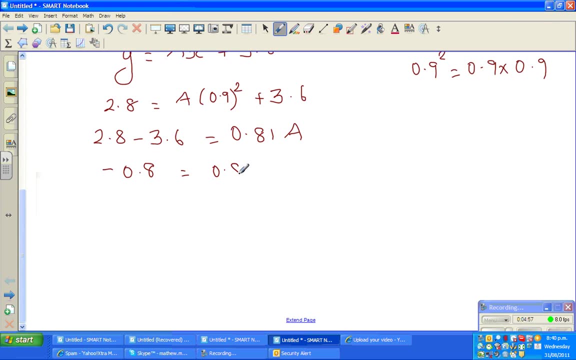 It's always good to check So menu. So 2.8 minus 3.6 is minus 0.8.. I was right. So minus 0.8 is equal to 0.81 a, Okay, Okay, And now I'm going to divide both sides by 0.81.. So A is negative 0.8 over 0.81.. Okay, and that's what I told you. it has to be negative. So again, let me get the calculator out. 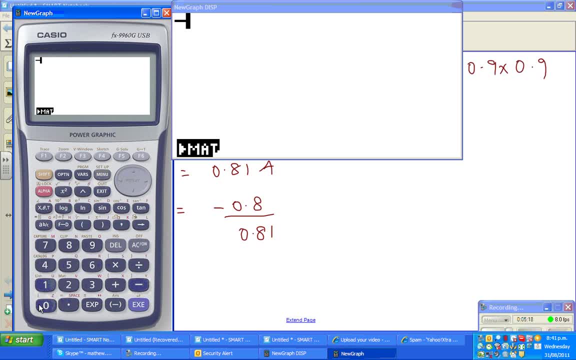 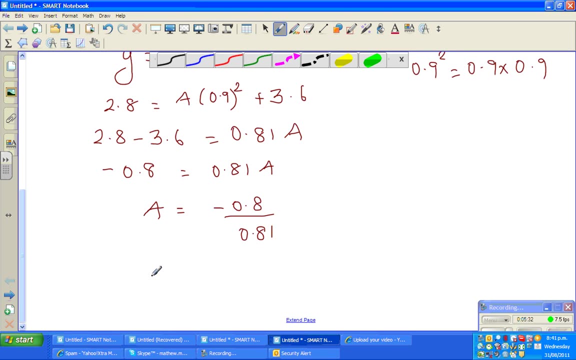 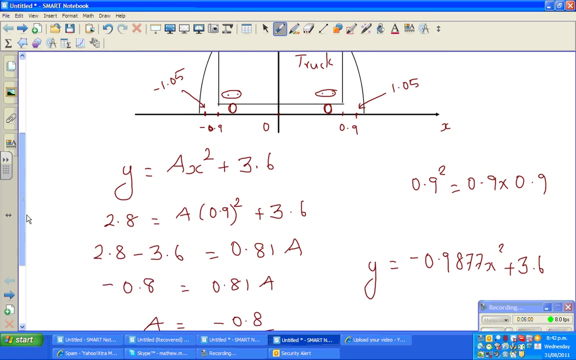 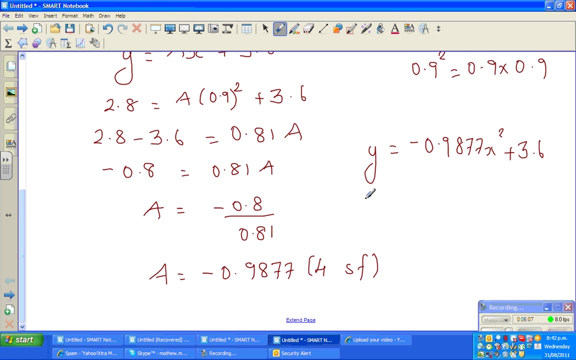 When you run. so negative 0.8 divided by 0.81 is 9877 in four significant figures, or four decimal numbers. So A is negative 0.9877 in four significant figures, Four significant figures, Four significant figures. Okay, So now the equation becomes: Y is equal to negative 0.9877, X squared plus 3.6.. Now my question is very simple: If X is 1.05, how much is Y? That will give me the height, So Y. so the question is: when X is 1.05, what is Y? 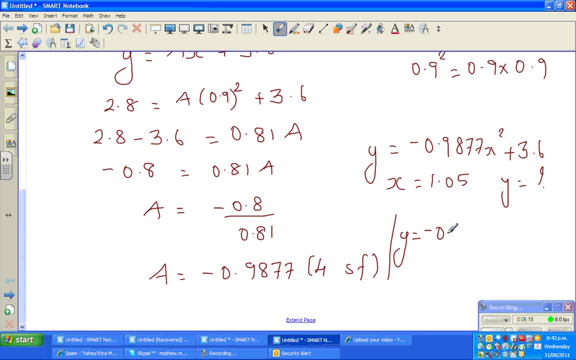 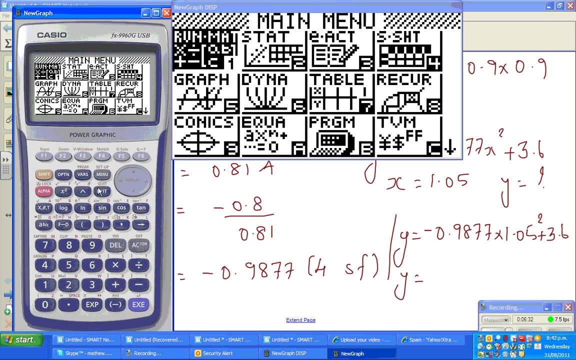 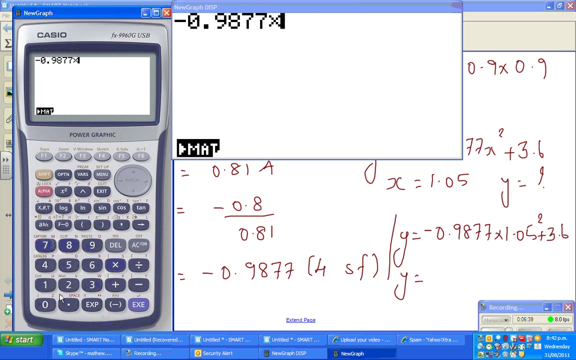 That's pretty simple. This is: Y is equal to negative 0.9877 times 1.05 squared plus 3.6.. For this I'll need a calculator. So let me get a calculator Menu run: negative 0.9877 times 1.05 squared plus 3.6.. 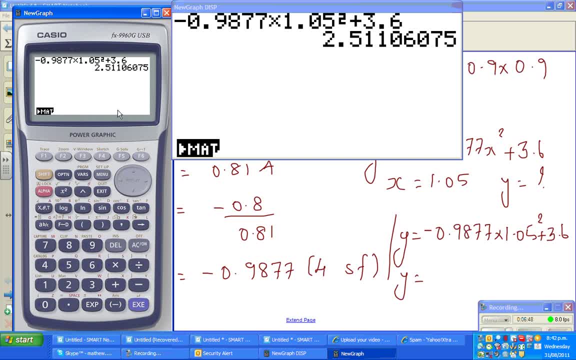 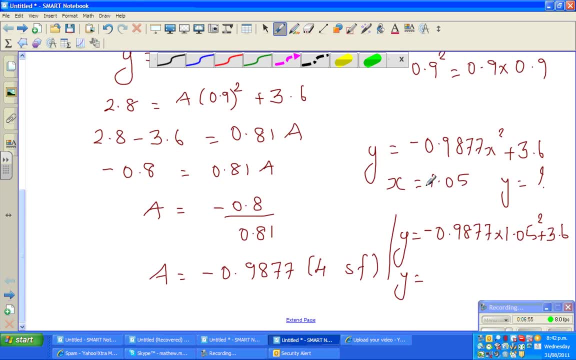 And here we go. The answer is 2.5 in one DP. Okay, or 2.5 meters. So that's the maximum height the truck can be. So this would be 2.5 meters in one decimal place. Okay. so this is your answer And if you can do this, you are getting- you would get- an excellence in your NC exam. Best of luck for your NC exam. That's a coming out. Thank you.